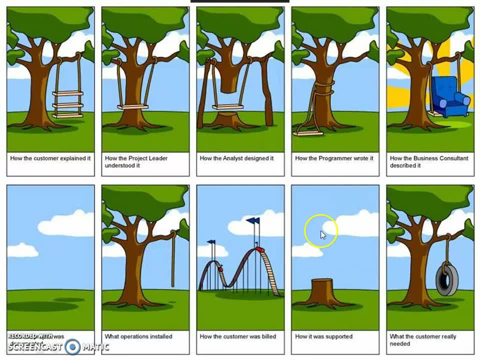 Well, you've got half the tree there, but not the top part. that's important, And then, ultimately, what the customer really needed. So, instead of a swing like this, what was really needed was a tire swing like this. So I include this because I think it's funny, but it's also perhaps indicative of the many, many ways that design processes work. 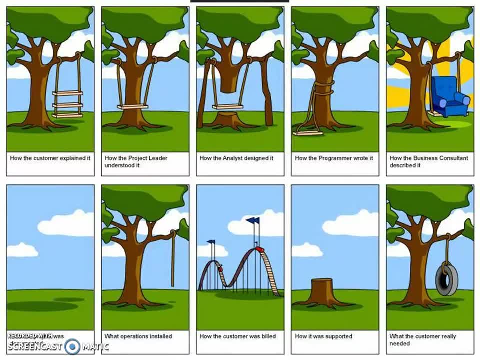 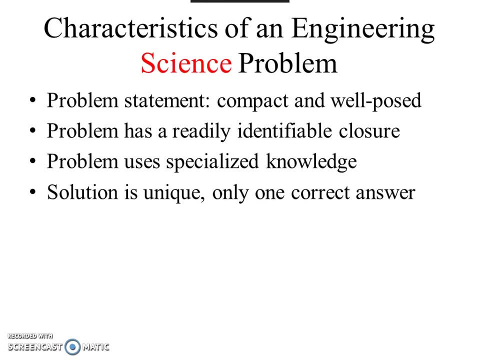 Particularly with large organizations, can go awry. So really the purpose of this course is to teach you guys the correct engineering design process to avoid a lot of the pitfalls in this comic. So really the place to start is to describe the difference between the characteristics of an engineering science problem and an engineering design problem. 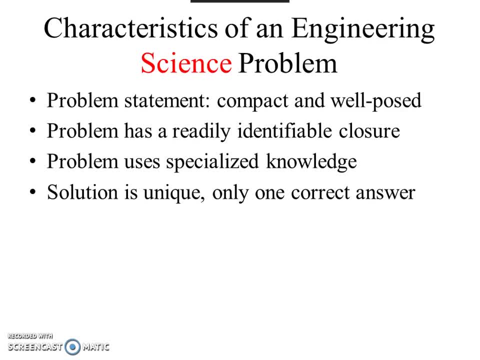 The reason that I start with this is because up until now you've been solving engineering science problems. So these are problems where you're given a problem statement, a paragraph. It's compact, well posed, well thought out. The problem has a readily identifiable closure. 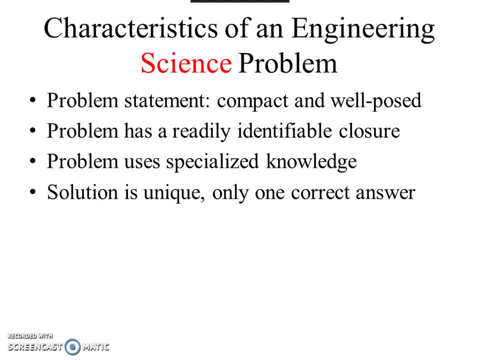 That means you can crank through some calculations and you can get to what seems like the end of the problem. There's no need to iterate again, to try to solve the problem again once you've solved it the first time. The problem uses specialized knowledge. 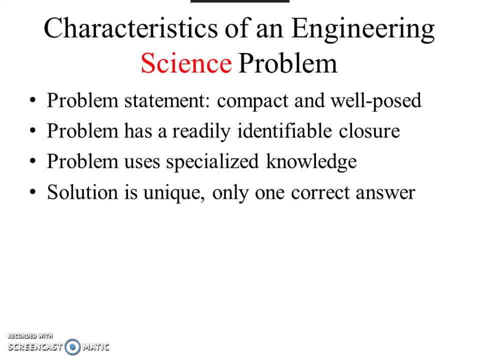 So you think of classes like controls, thermodynamics, heat transfer, fluid mechanics, manufacturing and so forth. That's the specialized knowledge that's required to solve problems in the engineering science domain, And then, ultimately, the solution is unique, in that there's only one correct answer. 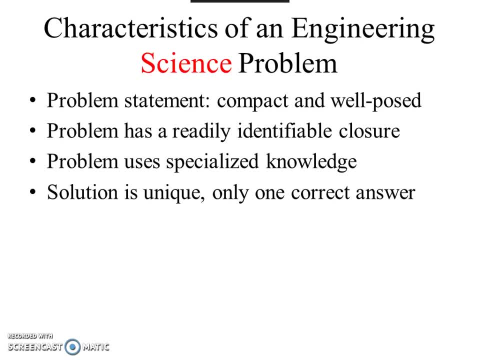 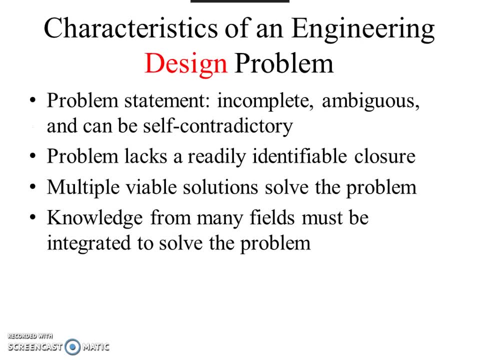 And once you get to that correct answer, the problem is solved And you don't really have to spend any more time thinking about it. By contrast, engineering design problems come with a problem statement, usually from a customer, that is often incomplete, ambiguous and even, at times, self-contradictory. 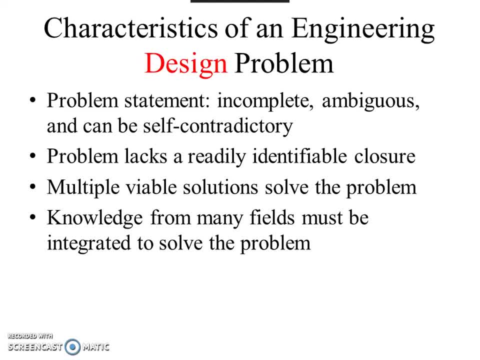 The problem lacks readily identifiable closure, meaning you can continue to improve to try to make a better design. You can iterate essentially forever And perhaps not get to the best possible solution. There's also multiple viable solutions to the problem, So you could find yourself going down one path only to realize that there's a better solution down some other path. 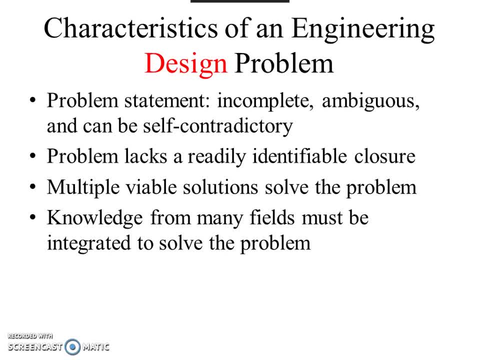 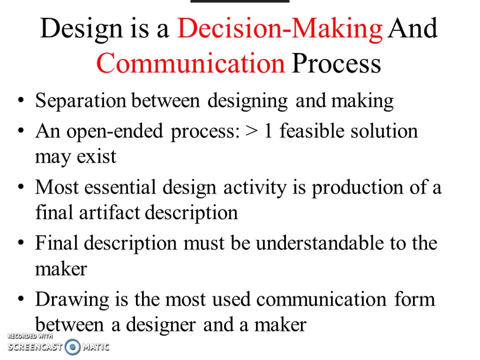 And those solutions. both might solve the problem, but one could potentially do a better job than the other. And then, finally, knowledge from many fields has to be integrated to solve these types of design problems. Design is also a decision-making process and it's a communication process. 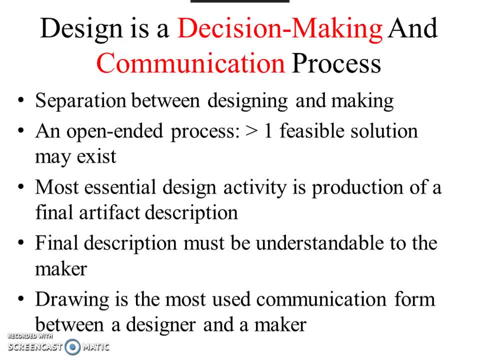 And the reason for that is because at least in the modern industrial world, there's a separation between the engineers who do the design and the technicians who do the making, the manufacturing. As I mentioned in the previous slide, design is an open-ended process. 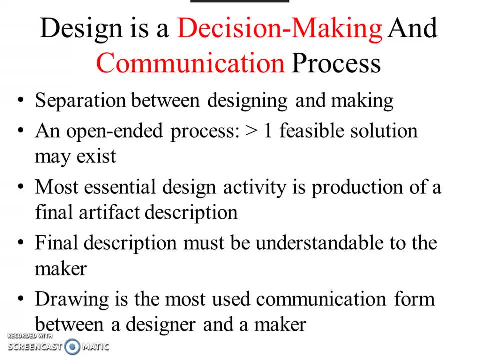 There's more than one feasible solution, And so if you just take the customer needs and you communicate the customer needs to the people who are making this product, who are manufacturing this product, because there are multiple possible solutions, it's not going to be clear to the people making the product how to make it, because there's many possible solutions. 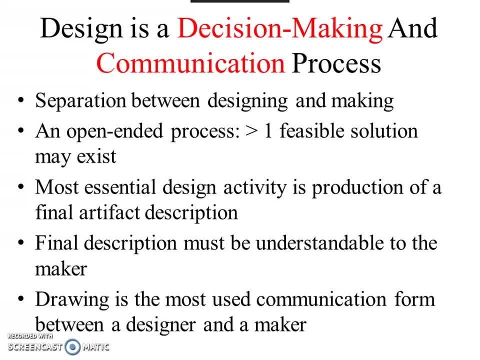 And so what's needed is a final artifact description, And that turns out to be the most essential. It turns out to be. the most essential activity of the design process is to come up with an artifact description And, importantly, that description has to be understandable to the people who are making or manufacturing the final product. 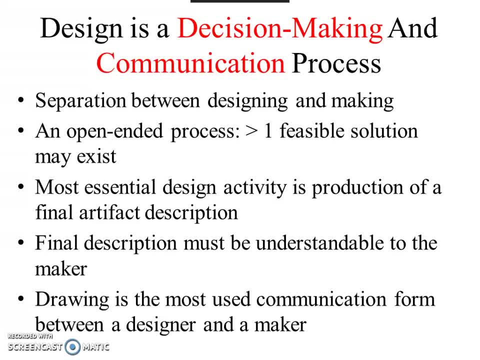 So typically in engineering we use technical drawing, engineering drawing as the most common form of communication between a product designer and a product maker, And that's why, very early in the engineering curriculum, you probably took a course in engineering drawing, so that you could learn how to make those images, those drawings that really communicate everything from the shape of the product that you wanted to make.